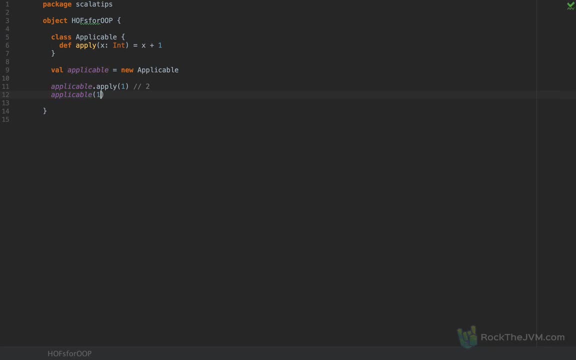 be invoked themselves. So something like this: applicable invoked with the argument one, And this is actually equivalent to applicableapply with the argument one. So the apply method allows objects to be invoked like functions, And so objects with apply methods like these can behave. 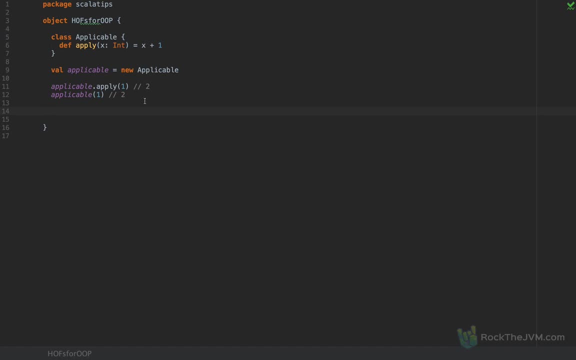 like functions. They take arguments and they return results. The Scala standard library actually has built-in types for function-like objects which are nothing else but plain instances with apply methods. Let me give you an example. So these are function objects I'm going to define. 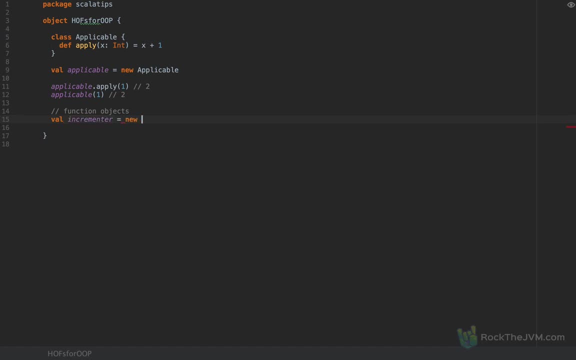 a value called- let's call this incrementer as new And I'm going to use the Scala standard type function one, And you notice that Scala has function all the way up to 21.. So function one with the types int and int, meaning a function that takes an int argument and returns an int result. 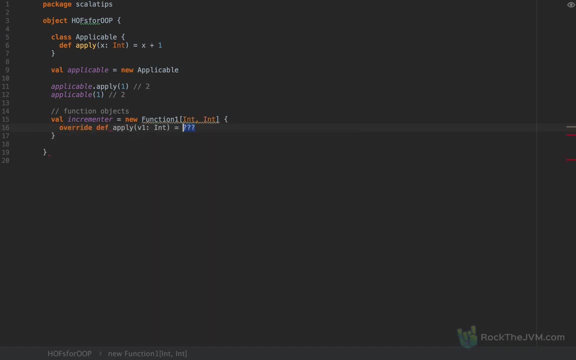 And this function trait actually has an apply method that I'm going to implement here on the spot. And given an x, I'm going to return x plus one. This incrementer is a plain JVM object, much like this applicable that I've defined above. So I can say, for example: 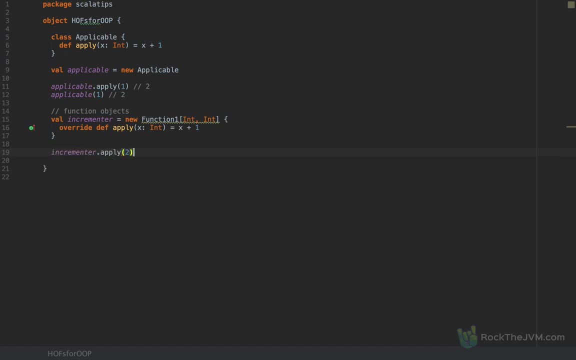 incrementerapply with the argument two, and I would return the value three. or incrementer invoked with the argument two and I would return three. Now, Scala being the nice functional language, it is allows for nice and concise syntax sugars. So I'm going to define a value. 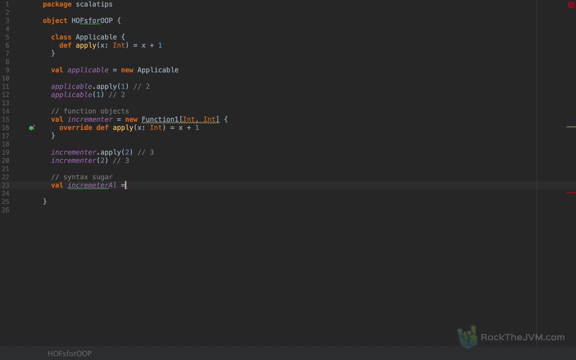 let's call this incrementer, alt as, and I'm going to use the shorthand notation x, colon, int arrow, x plus one, which is nothing else but a new function, one definition, And if you hover over this warning, syntactic sugar could be used. And if you define a lambda, an anonymous function, much like the way I did here on the 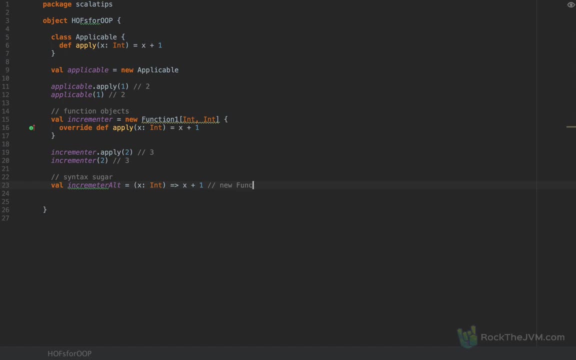 screen. this is actually equivalent to defining a new function, one with int and int whose apply method is whatever I wrote here on the right hand side of the arrow sign, And obviously this incrementer alt that I've defined also has an applied method. So if I said incrementer alt, invoked with the 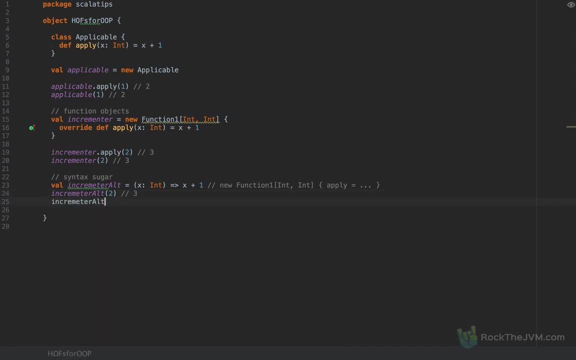 argument two, that will be three, and incrementer altapply with the argument two, that will also be three. Cool Now, naturally, because these so called functions are nothing but objects, with apply methods. they can be passed around as arguments or returned as results. So the functions. 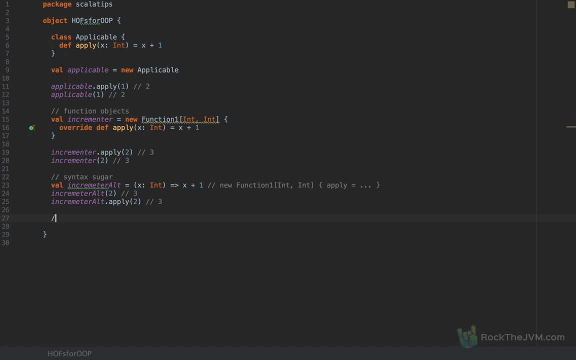 arguments or and or return other functions as results are called higher order functions, or Hoff's for short. So I'm expecting this to make sense for object oriented programmers. So these function objects in Scala are nothing else but JVM objects with apply methods, And this is 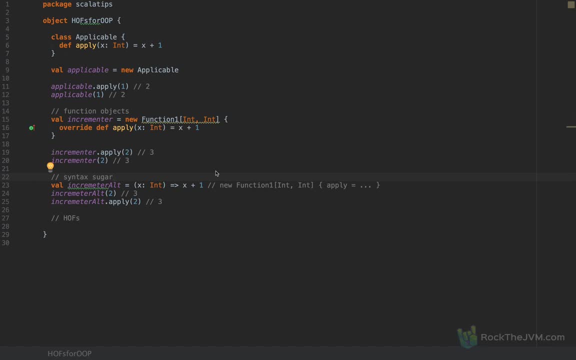 how the Scala functional programming paradigm is actually implemented on top of the JVM, which was primarily built for Java, which is an object oriented language. So this is how a functional programming language is actually mapped on the JVM. Now here's something I often ask people to do in my trainings. after the, I explain what I've already. 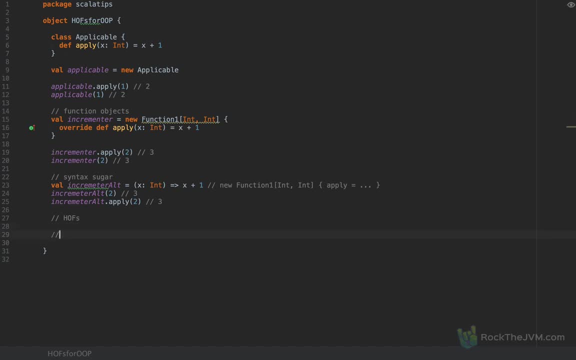 done here in this video. So let's go ahead and define an example or exercise, if you choose to take it. So let's define a function- I'm going to define that as n times, which takes a function, int, arrow int and the number n, which is an int, and returns another function of type int. 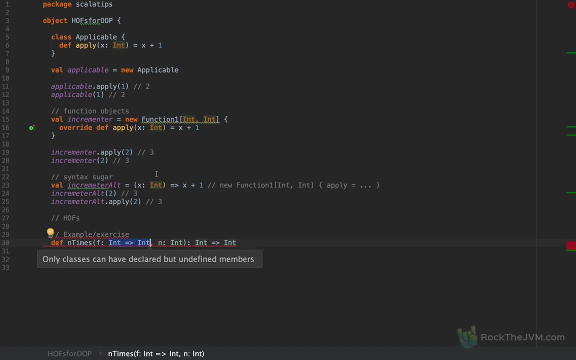 arrow int. The type int arrow int, by the way, is syntax sugar for function one, So there's nothing to rocket science there, And this returned function needs to have the following property: The function that I returned over here, applied to a certain argument, needs to invoke this function f n times. 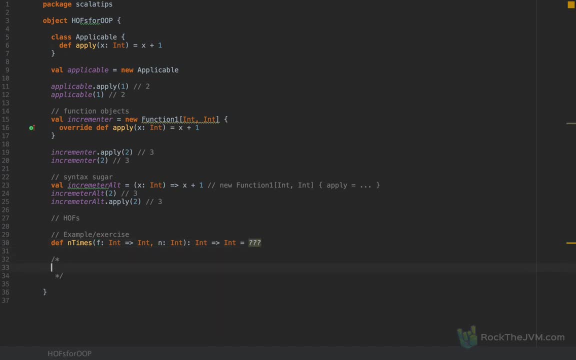 on this argument. So let's assume I have, for example, that's called. let's call this g. if I named g as n times with a function, f with the number 30, then g applied to an argument. let's call this g of x. 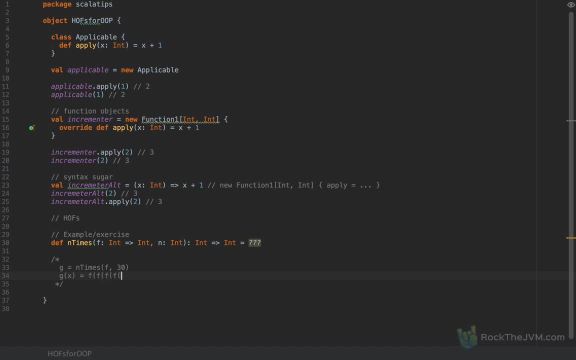 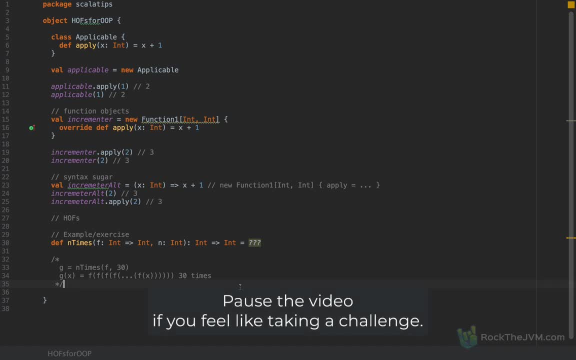 So if you want to take a challenge and implement this yourself, feel free to pause this video, And I'm going to write an implementation for this. So here's how I'm going to write this. I'm going to write as follows: I'm going to say: if n is less than or equal to zero, then I'm going to return a function. 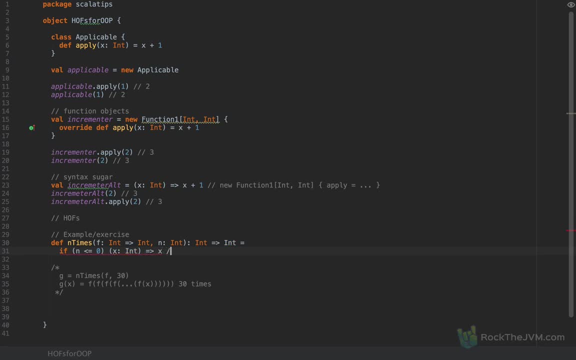 x colon- int arrow x. So this will be the identity function. Now, this is a function, because this is how I've defined the method to return. So I've defined the method to return a function- int arrow, int. And this is an object that. 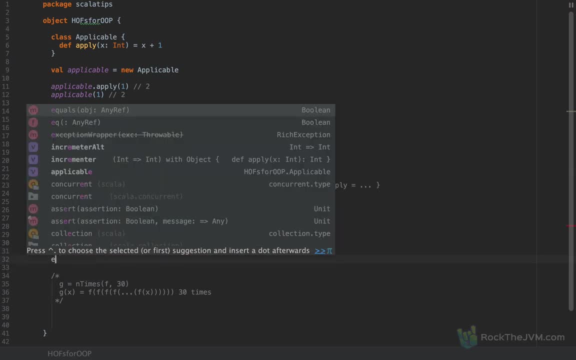 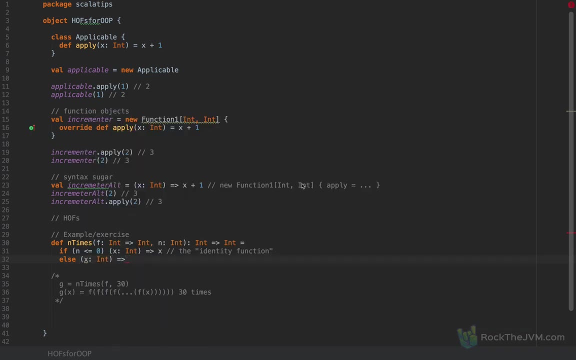 given an argument returns that argument. Otherwise, I will return a function that, given an argument, x arrow int, This function will return n times with f and n minus 1 applied to f of x. Now this is where people start to get a little baffled, because this code is very, very. 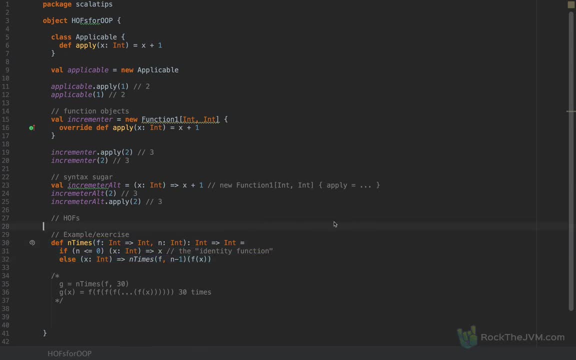 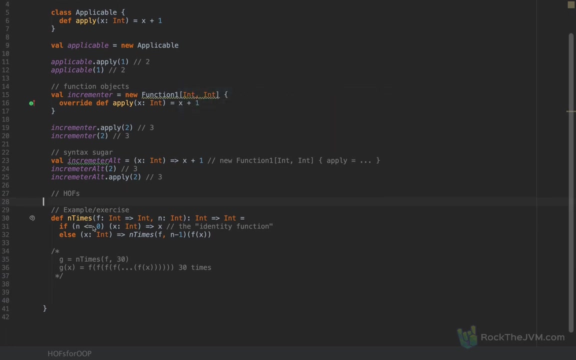 very concise. So this code is concise and often hard to read, especially if you've not done a lot of this before. So it's natural if it takes a few minutes to unwrap. So one of the questions that I asked first is: how do you read this in the first place? So let's take a look at the code. If n is zero or 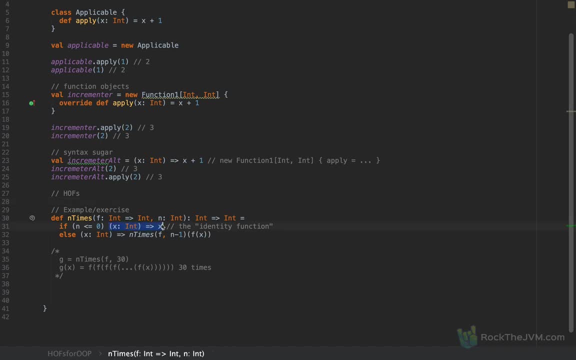 less. then we return a function that, given an argument, returns the argument. This is the identity function, which I hope makes sense. Otherwise, we return a function that, given an argument, applies the n minus 1 function onto f of x. So it's as if I said: apply to f of x. Now let's do a small breakdown. 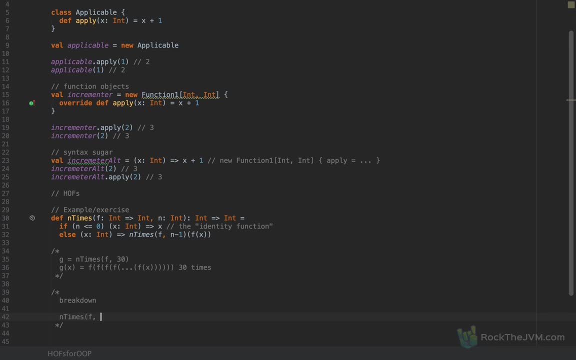 So if I wrote n times with f and 4, because 4 is not less than or equal to 0, then I will return x arrow, so x int arrow, n times with f and n minus 1,, so f and 3,. 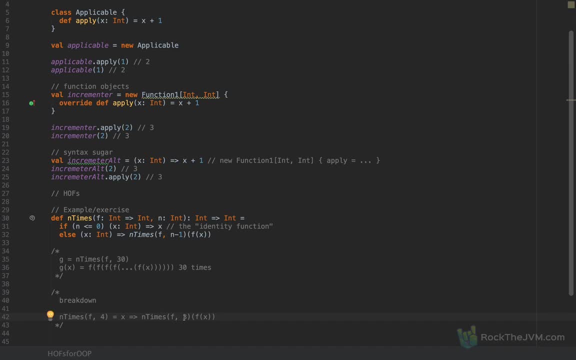 apply to f of x. Now, what is n times of f and 3, applied to f of x? So let's compute n times of f and 3.. This is x arrow n times with f and 2, applied to f of x. Similarly, we could write: 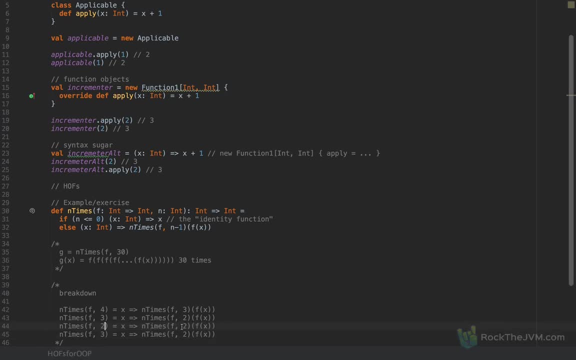 n times with f and 2 is x. arrow n times with f and 1, applied to f of x. And n times with f and 1 is x. arrow n times with f and 0, applied to f of x. 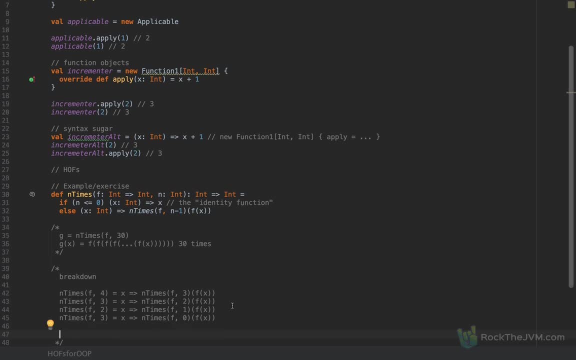 By the same mechanism. Now, what is n times with f and 0?? Well, n times of f and 0 is the identity function. that given an argument returns that argument. So that is x arrow, x. Well, given that n times of f and 0 is the identity function, let's apply that recursively backwards. So n times of f and 0 applied to this argument. 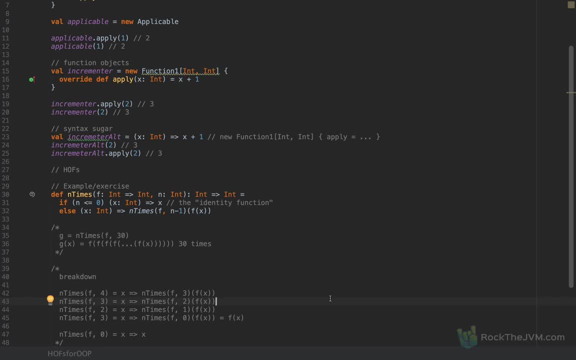 returns this argument, so f of x. So we can say that n times of f and 1, I've mistaken here. so n times with f and 1 is a function that applies f to the argument. So n times of f of 1 is x arrow f of x. Let's re-raise that: So n. 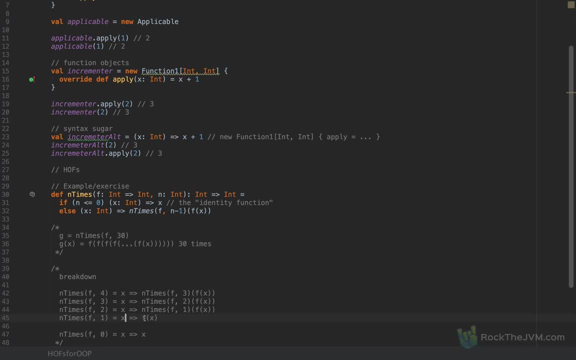 times of f and 1 is a function that, given an argument, just applies f to that argument. Cool, now let's use this over here backwards. so n times of f and 1 applied to f of x, is f applied to the argument which is f of x. 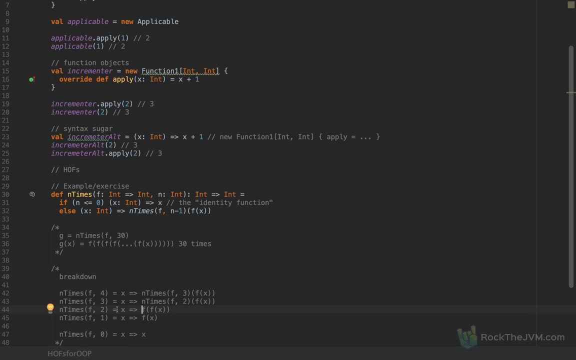 Let's erase that as well. So n times of f and 2 is a function that, given an x, applies f twice to the argument. Now, given n times of f and 2, we can actually apply that here. So let's invoke an apply, and that would be f applied to. 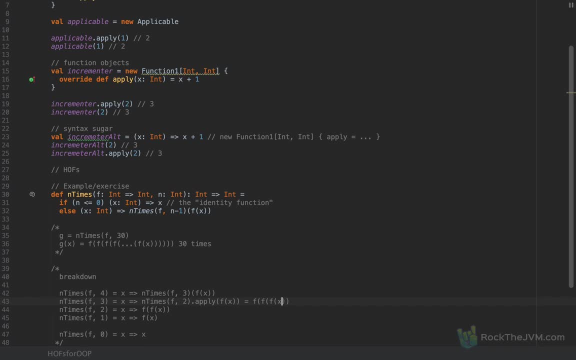 to f apply to the argument, and the argument is f of x. So notice that we now have n times with f and 3 applies f three times to the argument. and in a very similar fashion, we will obtain n times with f and 4 applies f four times to the argument. So this will be f. apply to f. apply to f. apply to. 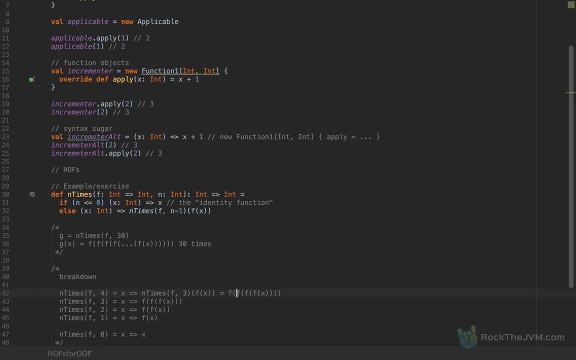 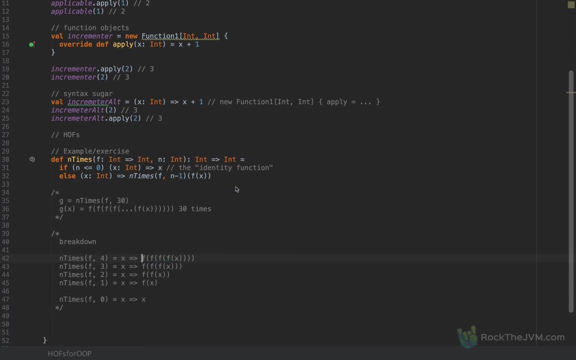 the argument f of x. So this will be the breakdown of how this function will actually work. Cool, so that is how we read and we break down the implementation of this function. If you want, you can pause the video and take a couple of minutes to actually break this down. 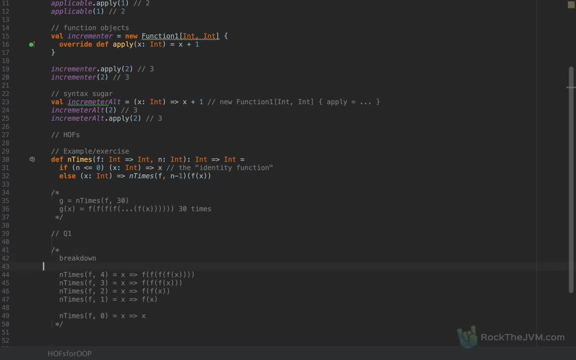 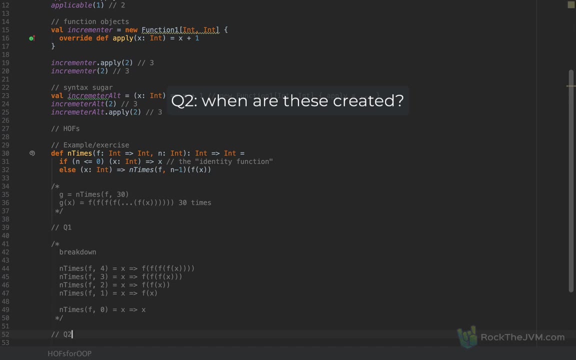 yourself. So that was q1.. Now for question two. that I often ask a lot is: when are these functions actually created? If we read the code, we can see that all these intermediate functions over here are not actually created until we actually invoke the result function. So for 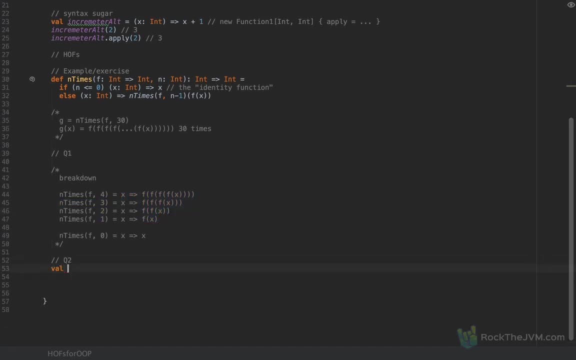 example, if I said: let's call this val, let's call this f4 as n times with f and 4, and let me define an f. let's call this x int arrow, x plus 1.. Okay, and I've defined an f4 as n times with f and 4.. Well, 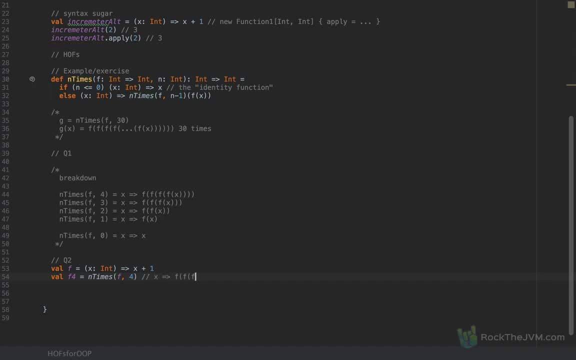 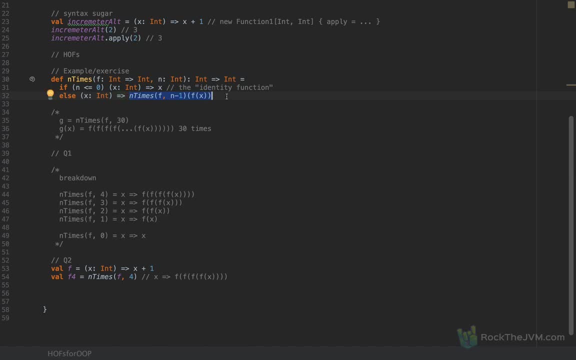 x colon int arrow n times with f and 3 applied to f of x. It's as if I said: let's call this f4 alt as x colon int arrow n times with f and 3 applied to f of x. So this will be a single object. 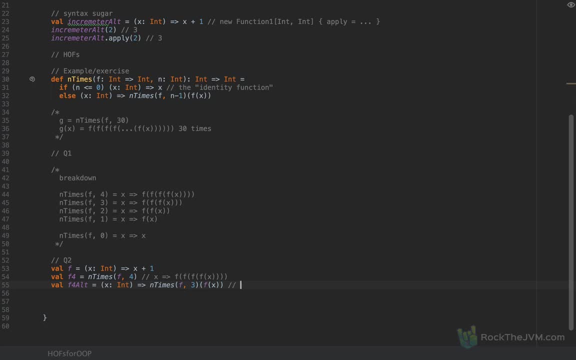 not multiple functions, intermediate created. So it's as if I said: new function 1 with int and int, in which the apply method is actually n times with f and 3 applied to f of x. So notice, a single object is being created here from a JVM perspective. 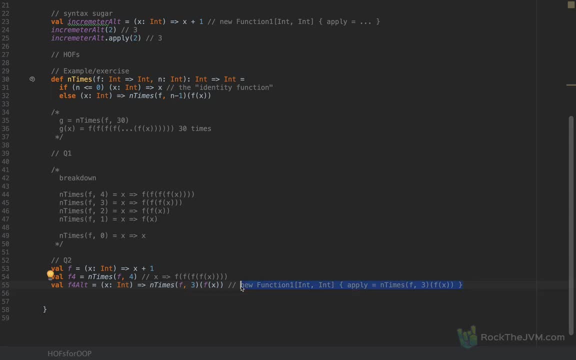 So from an object oriented perspective, a single object will be constructed. On the other hand, if I called f4 of 5, so if I invoke f4 with a real argument, then all the intermediate functions, n times of fn1,, n times of fn2,, n times of fn3 and n. 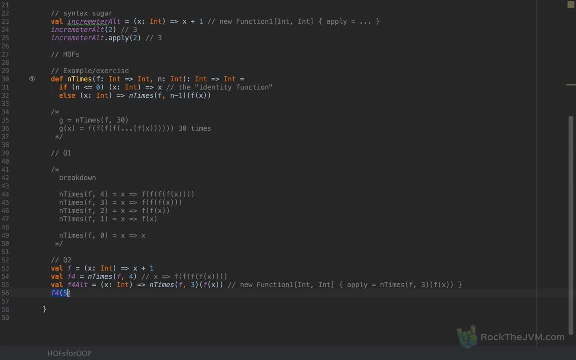 times of fn4 will be created so that I could invoke f4 of 5.. So all the function objects will be created for this particular case. So that was for question number 2.. Question number 3 is okay, Daniel, I understand the mathematical definition. I understand. 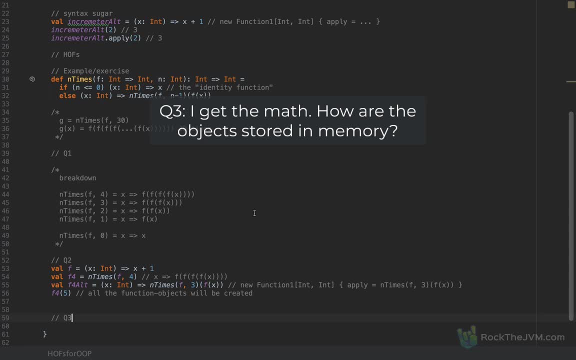 this recursion. but to an object oriented programmer like me, how are these functions actually created in memory? Because I understand how these functions are being applied and I can understand the recursion. but where are these functions actually stored in memory? How should I think about them in an object oriented fashion? 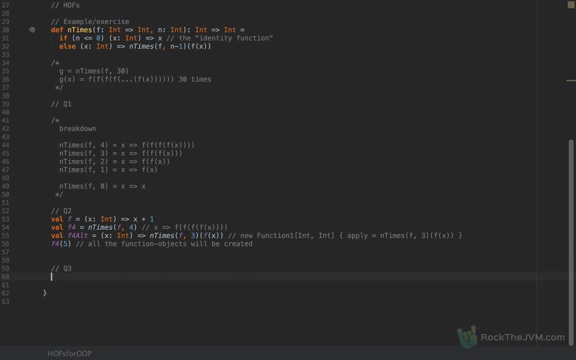 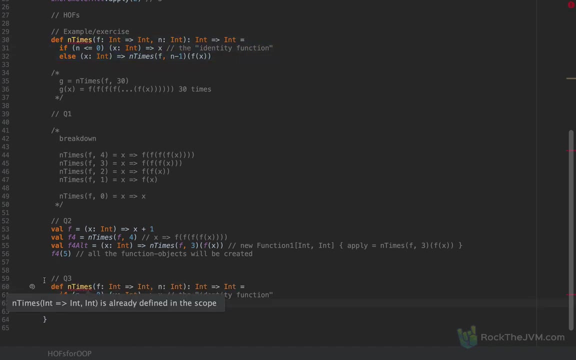 So it's worth coming back to the origins of functions that I've explained above. So let me rewrite the code with the original types, Let me copy this method n times and I'm going to call this n times original. And instead of the sugar types, int, error, int and all these recursive implementations. 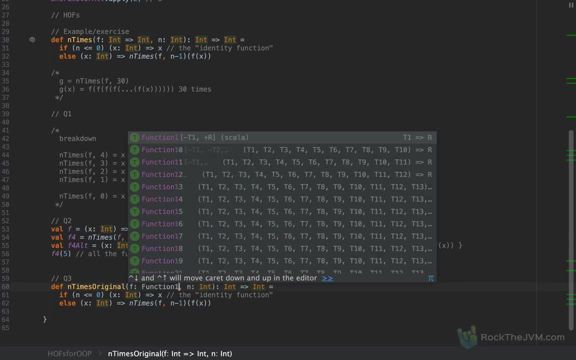 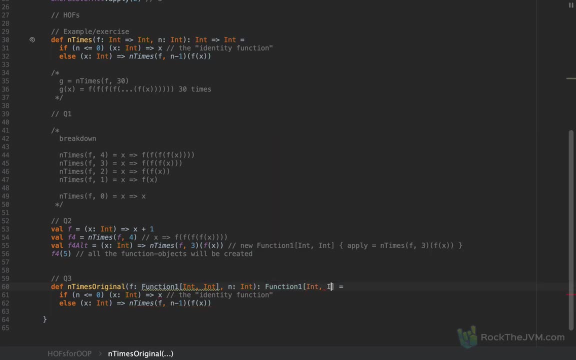 I'm going to use the original types. I'm going to use function1 with int and int And this will be another function1 of int and int which, in terms of Java these are only interfaces. So this function1 is a trait in Scala which to a Java programmer is equivalent to an interface. 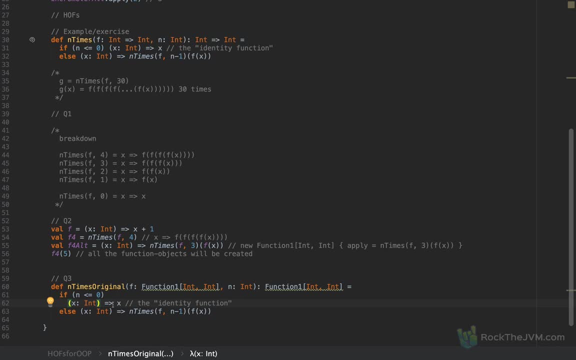 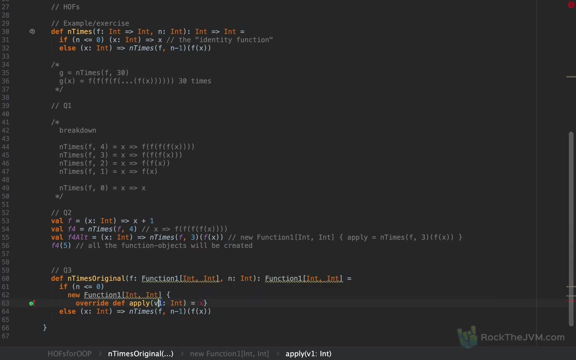 So, instead of x error x. colon int error x, I'm going to return a new function1, in which, with the int and int types in which the def apply, Look, It looks like x. Let me arrange the code so that you can read it better. 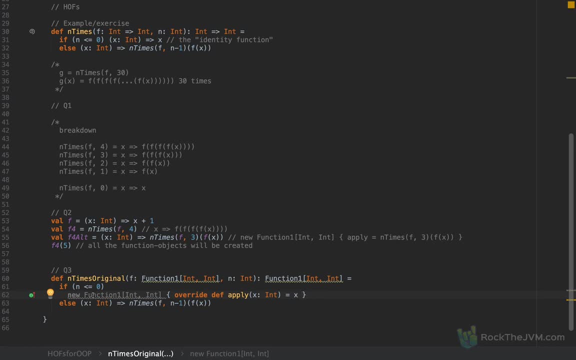 So if n is less than or equal to zero, I'm going to return one of these function1 types in which the apply method takes an argument and returns that same argument. So this is a JVM object. In the exact same fashion. instead of this error function, this lambda, I'm going to 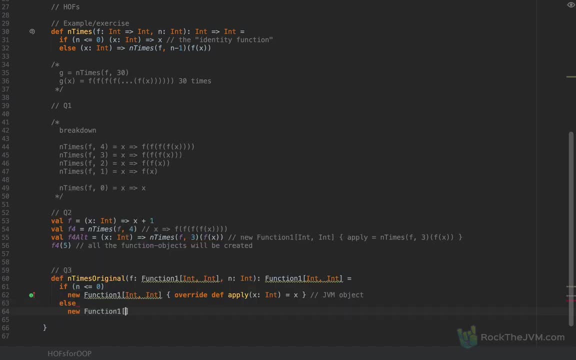 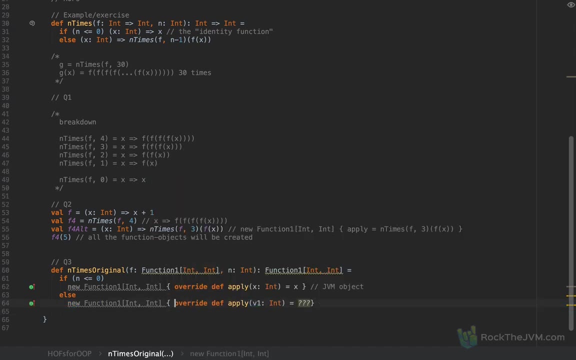 return a new function1 with int and int And I'm going to call this function1.. And I'm going to call this function1 with int and int, in which the def apply method takes an argument. Let me arrange the code So: the apply method takes an argument and, as an implementation, it returns n times original. 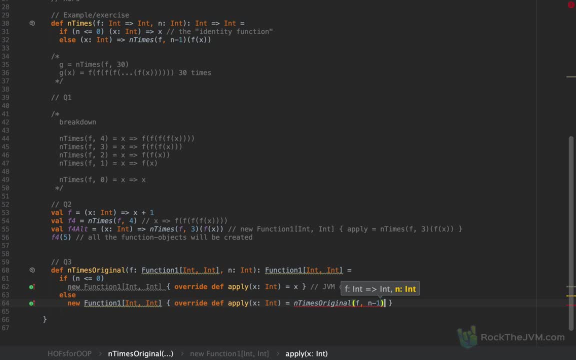 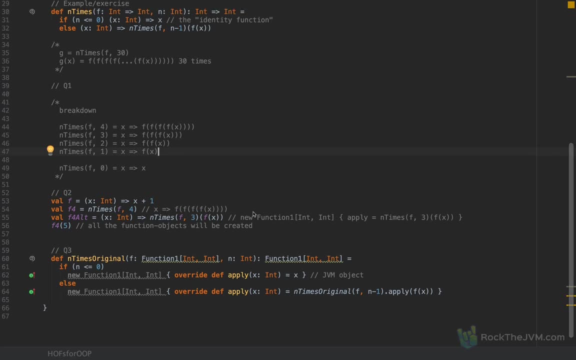 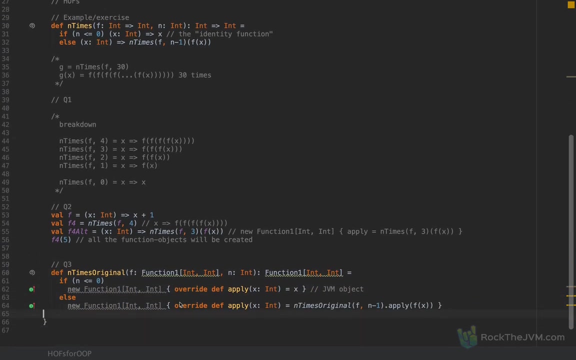 with the same function and n minus 1, applied to f of x. Now, somewhat counter-intuitively, it's easier for object-oriented programmers, and especially those with a Java background, to read this code- This code, as opposed to the previous one, which was more concise. 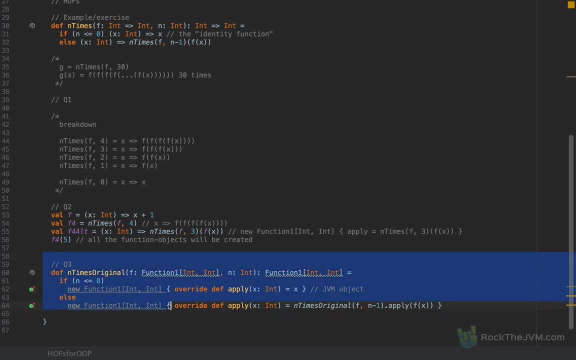 Whereas the more experienced you are with Scala, the more bloated this code will seem, because it has the explicit function types and Scala programmers like to be concise. If you come from a very heavy object-oriented background, this code will shed some light. 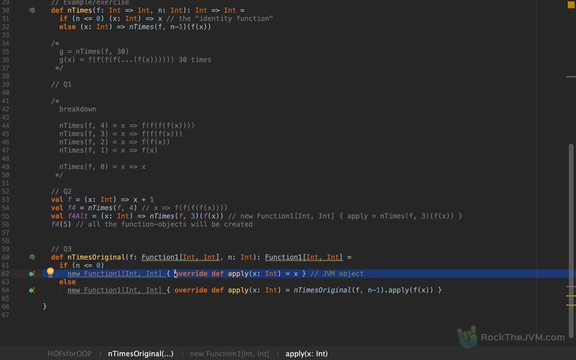 onto how the functions are being created as JVM objects, because we're now talking about plain JVM objects, not necessarily as functions, And if you track this down in the same style that we saw above, Like here, You will see how the function objects are being spawned in memory. 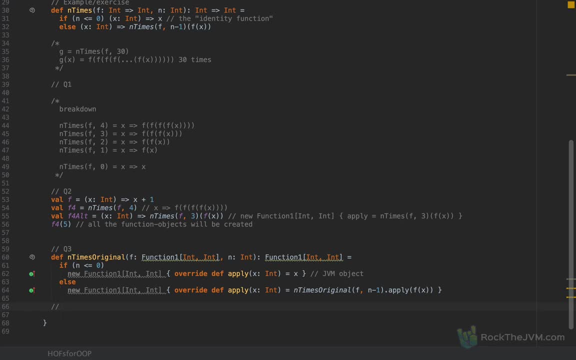 Now, immediately after that, a question that I get often asked is: isn't this using too much memory? Now, this question will take a short answer. Because this function is recursive, it will create a bunch of these function objects, but these function objects are very light because they only contain a small apply method. 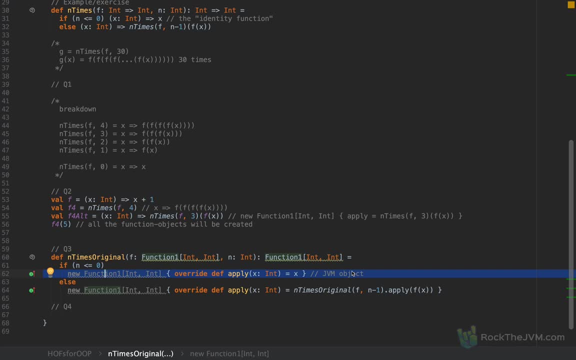 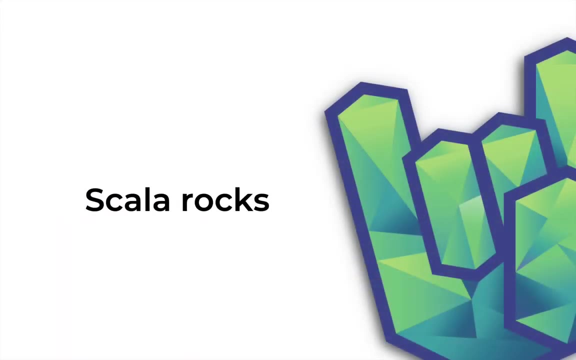 and they're also very short-lived, which makes them illegible for garbage collection from the JVM. so they will be quickly cleared. So I hope that will address the memory concerns. Alright, so I hope this was useful. I'm Daniel and you can find this article at rockthejvmcom forward slash blog. in written.